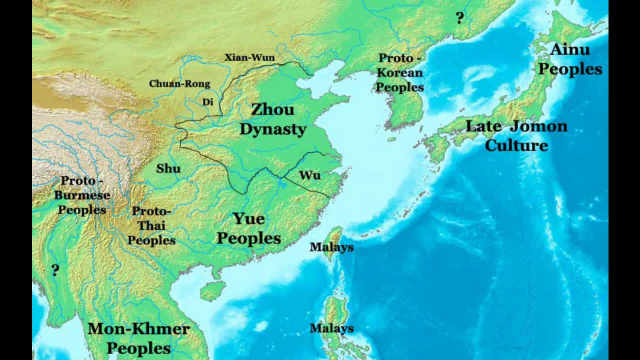 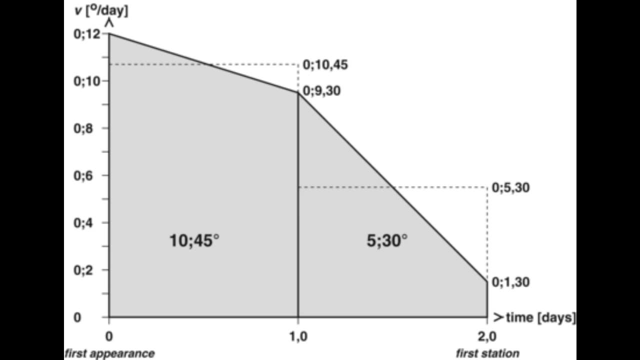 China. Most people that are familiar with the history of calculus know that the Babylonians had a primitive method of finding area underneath a line more than 1,500 years before Newton and Leibniz. Personally, I think the origins of linear algebra are even more astounding. 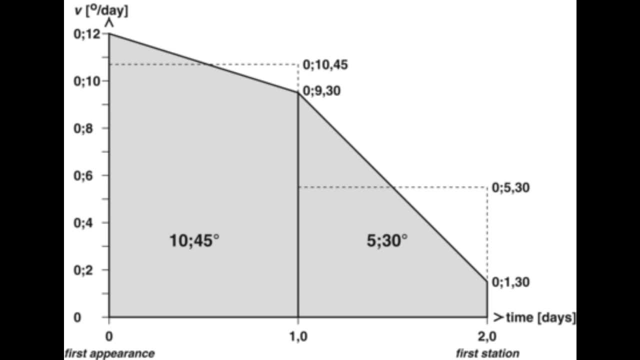 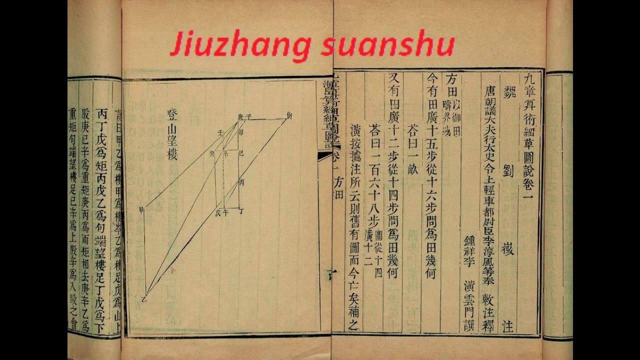 especially considering they happened even earlier. Between the 10th and 2nd centuries BCE, several generations of ancient Chinese scholars collaborated on a book known as Juzang Xuanzhu, or The Nine Chapters on the Mathematical Art, also known simply as The Nine. 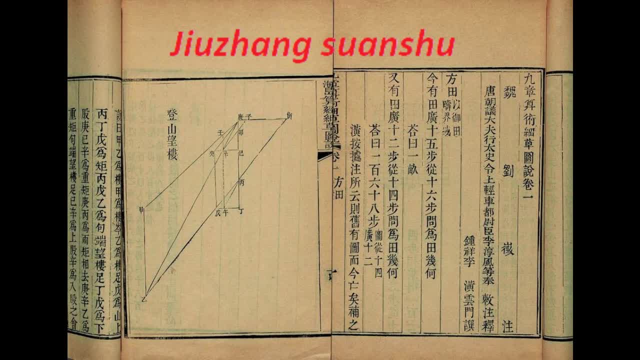 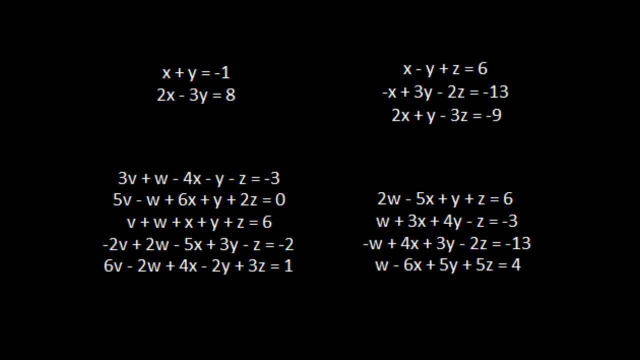 Chapters. In chapter 8, it lays out a method for solving systems of linear equations with two, three, four and five unknowns and equations. This method, called feng chang, is essentially what is known today as Gaussian elimination. They used counting rods to perform these calculations. 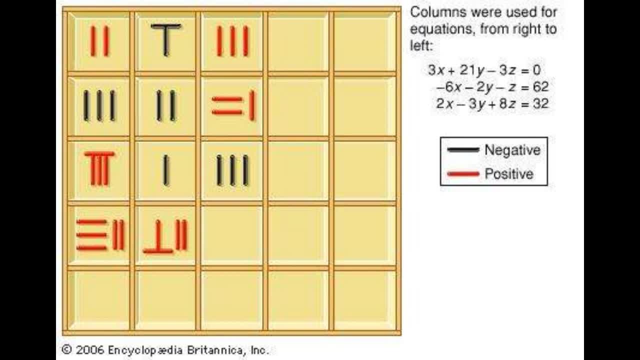 and the equations were represented vertically instead of horizontally, but the method itself will be extremely familiar to anyone who has learned row reduction. Problem 1 in chapter 8 goes like this: There are three different qualities of grain: high, medium and low. Three bundles of high quality. two bundles of medium quality. 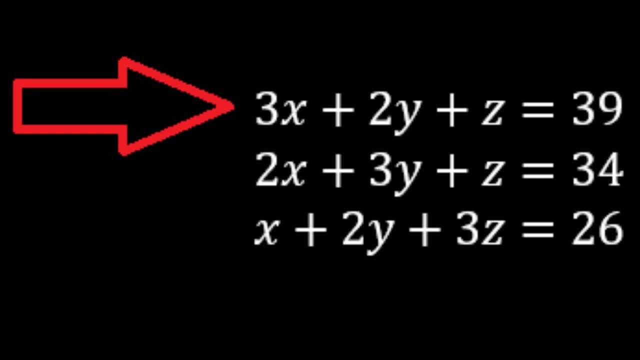 and one bundle of low quality grain gives 39 dao a unit of volume. Two bundles of high quality, three bundles of medium quality and one bundle of low quality gives 34 dao. One bundle of high quality, two bundles of medium quality and three bundles of low quality gives 26 dao. 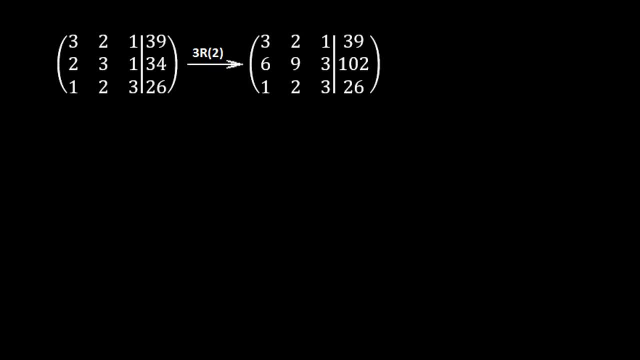 To solve for the amounts of each quality of grain, the middle row is multiplied by the value of the first value in the first row and then the first row is subtracted from the first row. The first value in the second row is zero. The process repeats for the first and third rows. 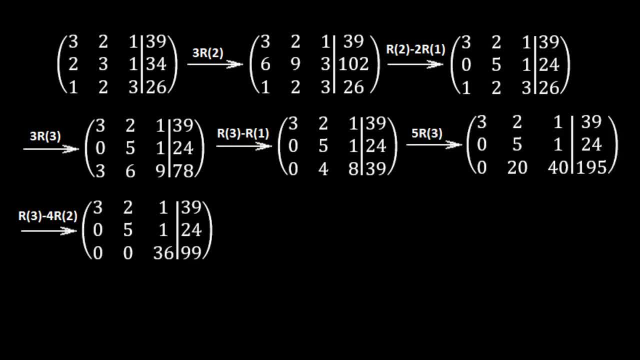 and finally the second and third rows with respect to the second value, since the first is already zero. From there, it's straightforward to calculate the value of the third variable, which can then be used to find the value of the second variable, and the two combined can be used to find the value of the first variable. 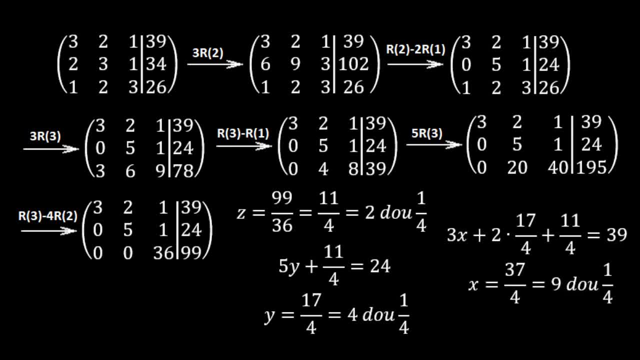 It's pretty easy to see how this method is essentially identical to Gaussian elimination, but this is what we're going to do next. This is where the development of linear algebra would sit for over one and a half millennia until the 17th century. In the early 1600s, René Descartes paved the way for the future. 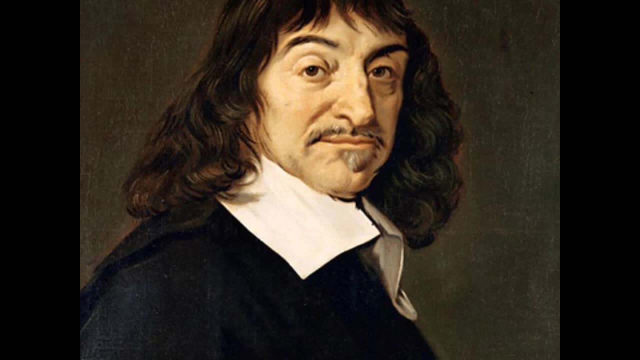 of mathematics with his development of analytical geometry. Before Descartes, mathematicians usually thought about math and calculations geometrically, providing visual proofs for algebraic concepts. Descartes viewed math the opposite way, in that he wrote his equations to fit their geometric. 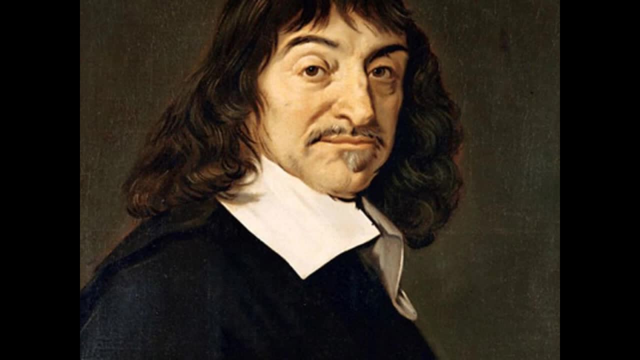 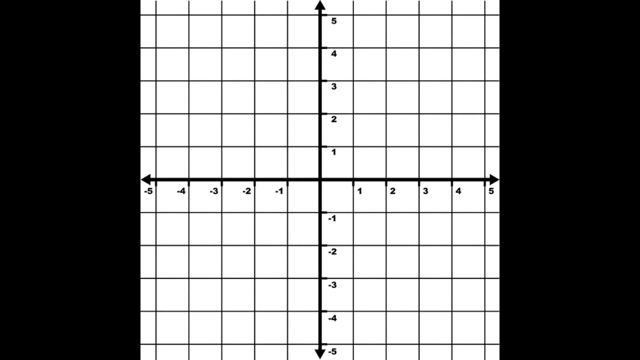 representations. This can be considered a turning point in mathematical history, where we started to think about math more abstractly and not necessarily something that has to be able to be represented in the physical world. He introduced the Cartesian coordinate system, which is ubiquitous in geometry today, and he began the tradition 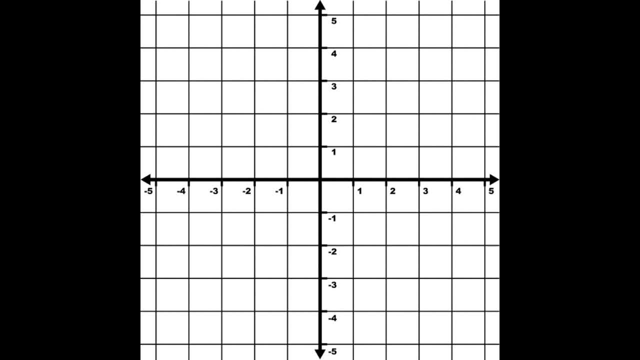 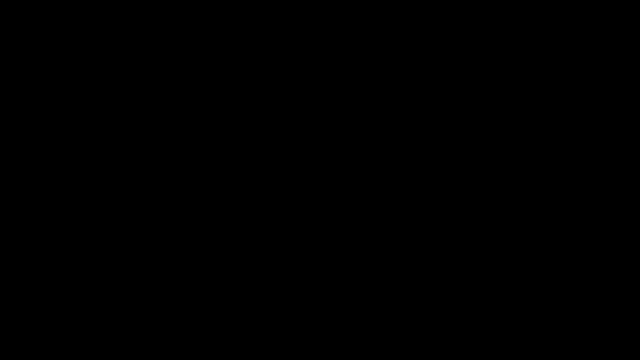 of using x, y and z to represent unknowns in equations. These developments are mathematical cornerstones and without them it would be extraordinarily more difficult to visualize. One of the first modern ideas of linear algebra to be discovered was the determinant Geometrically. 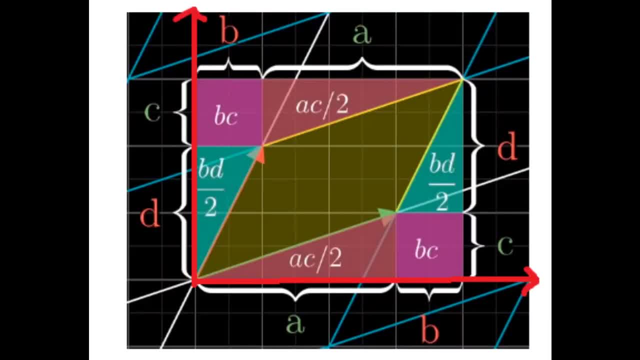 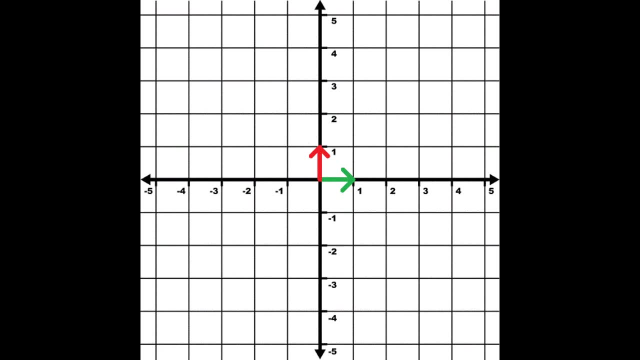 the determinant tells us the area or volume of the region bound by the unit vectors after a linear transformation occurs. so if the determinant is zero, the transformation can be thought of as squishing the vector space into a lower dimension. This means that the determinant allows us to find out relatively easily whether the determinant is zero or not. 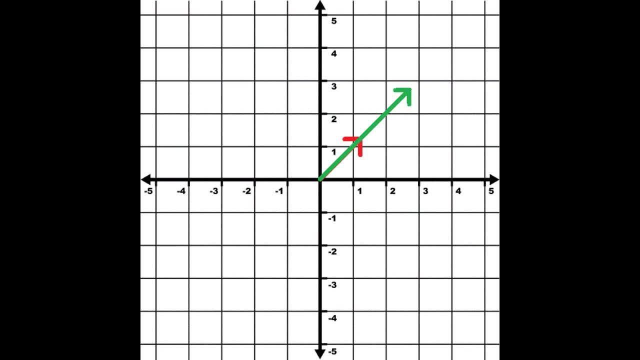 Whether a system of equations is linearly independent or not. If a system of equations is not linearly independent, at least one of the equations in the system lies along the same line, plane or other n-1 dimensional structure that is made by other equations in the system. 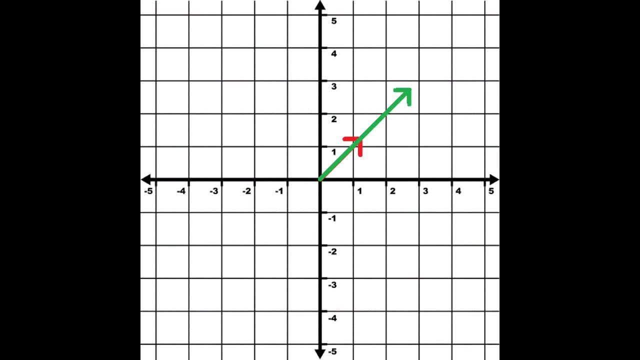 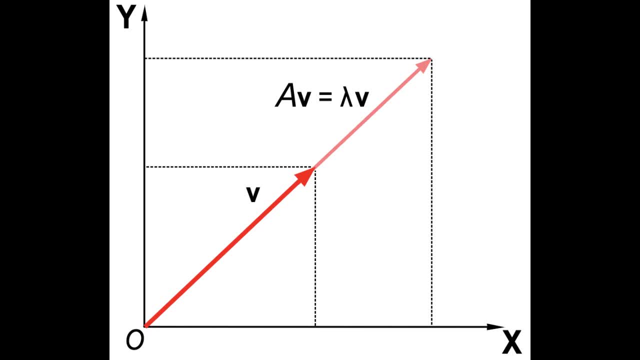 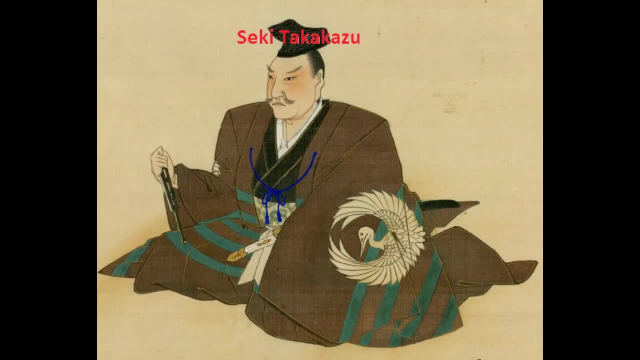 and can be described by using a combination of those equations. The determinant is also needed to find the eigenvectors of a transformation, the vectors which are only affected by a given transformation in magnitude. The Japanese mathematician Seki Takakazu, who some 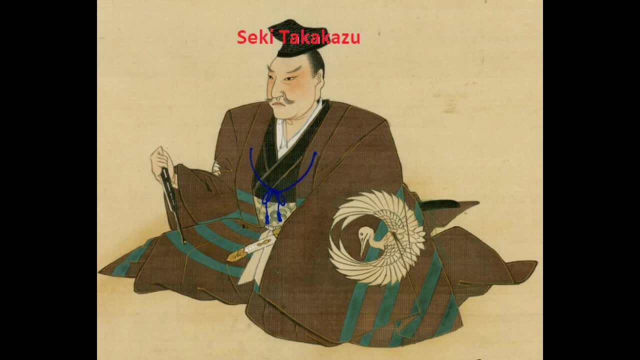 consider to be Japan's. Newton was the first to document the determinant in his book Taisei Sankei, which was originally published in 1683 and had editions made to it until 1710.. A European contemporary of his was also making progress in the discovery of the determinant. 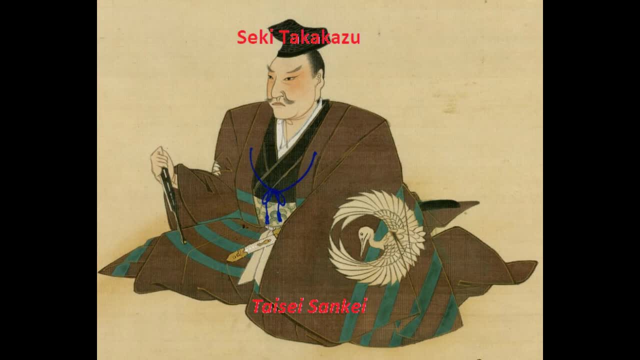 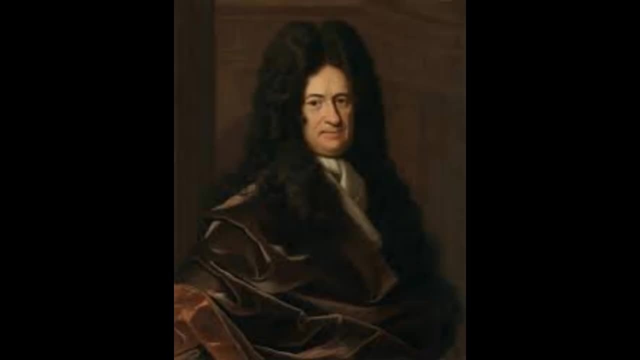 and its important properties, one who had a much greater opportunity to correspond with other mathematicians who were interested in the same problems. While Gottfried Leibniz is most known today as having independently invented calculus and developing the notation that is still used for it, he also independently discovered the 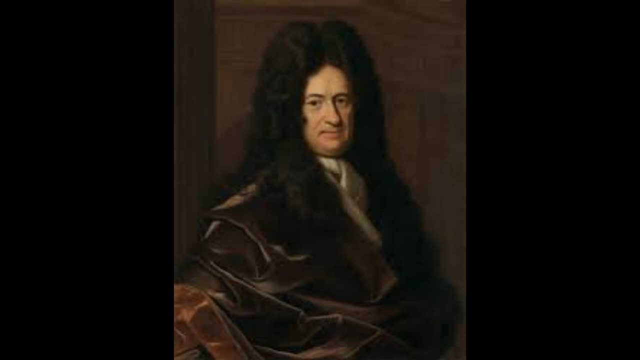 properties of the determinant. In a 1693 letter to Guillaume de L'Hôpital, he explained how he would sometimes use special notation to represent the row and column of a given value in systems of equations. He also explained how a given value can be used to represent the row and column of a given value in systems of equations. 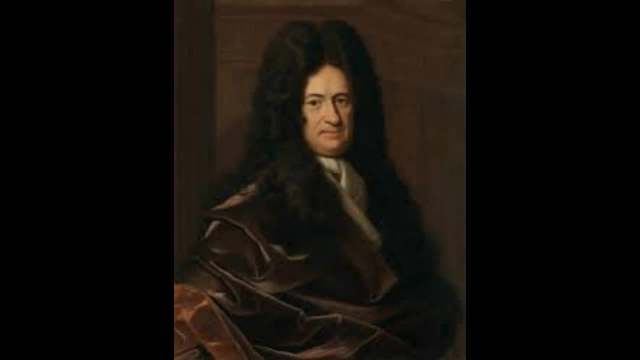 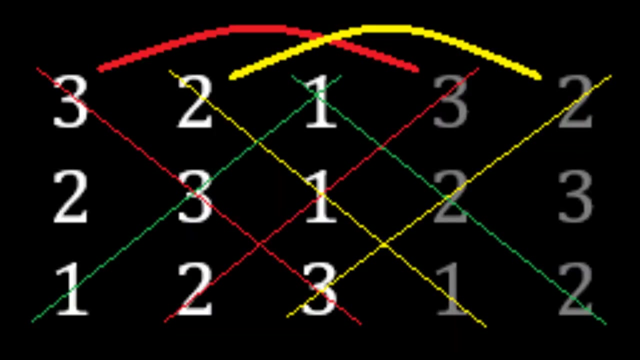 He would use this notation to represent coefficients in the form of an array, which eventually turned into matrix notation. From there he discovered that multiplying values along diagonals of the array that are rooted at the same value in the first row would equal each other. In other words, he was finding systems of equations whose determinant was zero. This was 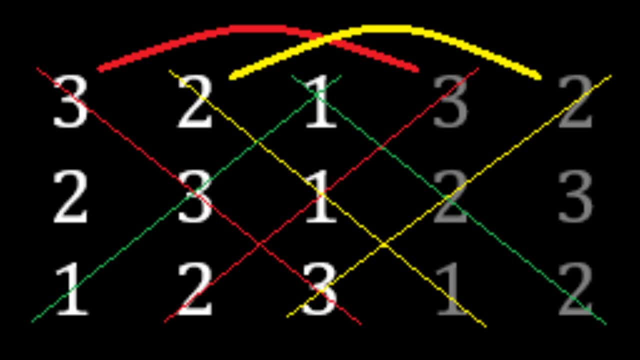 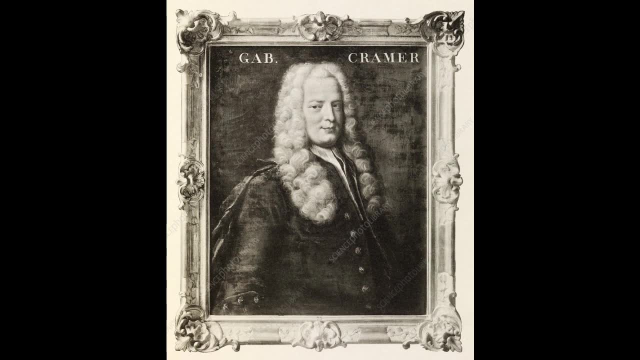 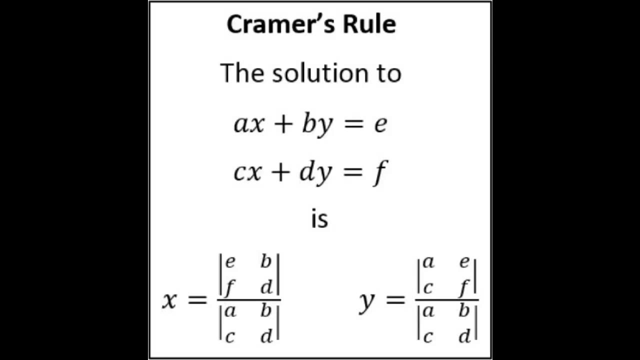 called the Leibniz formula for finding determinants. However, his discoveries weren't published until 1850, and it was Gabriel Cramer who found a way to solve systems of linear equations using the determinant. In 1750,, he published what would be known as Cramer's Rule. If the system of 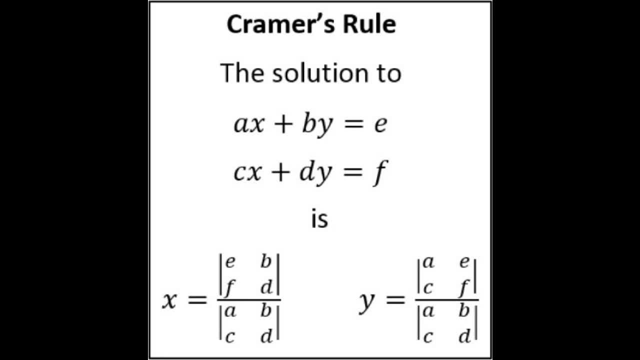 equations has a unique solution, then the unknowns can be found by only using determinants of given values. The value of each variable can be found by replacing the matrix column representing that variable with the values on the right-hand side of the corresponding equations and dividing the 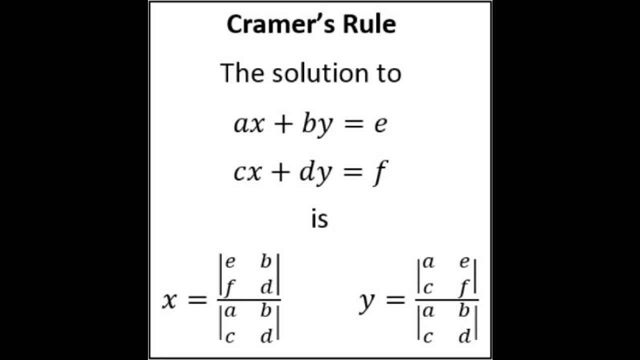 resulting determinant by the determinant of the original matrix. This method can be useful when there are only two equations and unknowns to solve for. but as more equations and unknowns are added to the system it can become very cumbersome to find all of the determinants. Gaussian elimination. 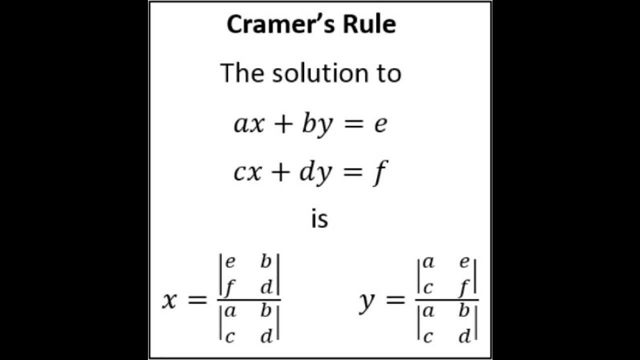 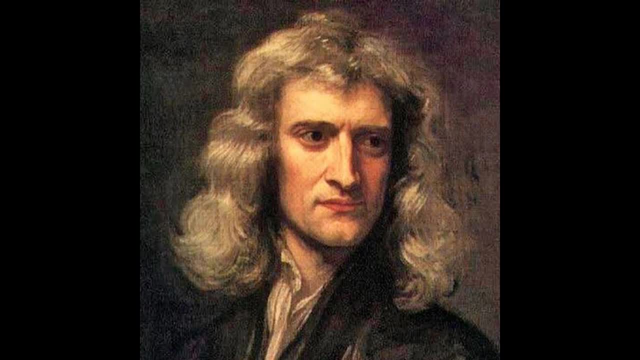 had been rediscovered about 40 years prior to Cramer's publication, but not by who, you would think, Despite the name. it was actually Isaac Newton who rediscovered the method used in the nine chapters to solve systems of linear equations. His notes, which explained this method, were published. 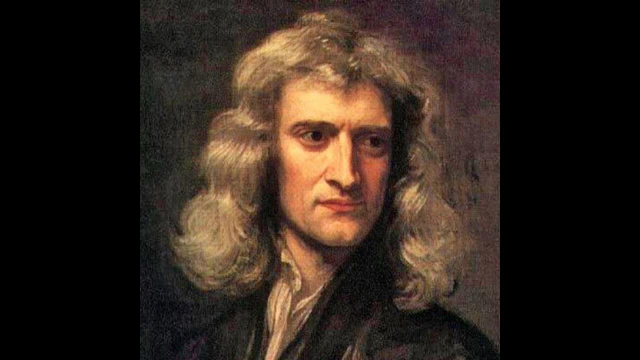 in Latin in 1707 and in English in 1720.. Over the following 80 years, this system of elimination of variables became well known due to its relative simplicity, only requiring a passing knowledge of algebra to solve equations that fit a square matrix. 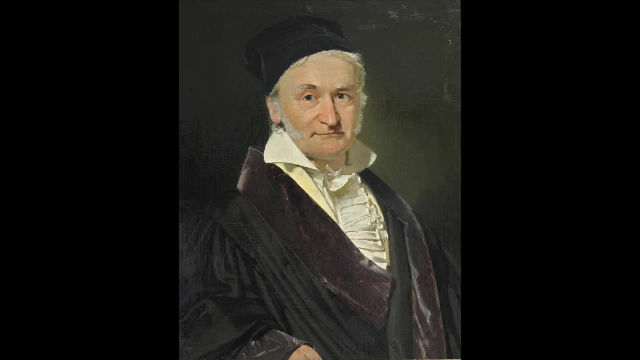 The method is attributed to Carl Gauss, because he used it extensively in his study of planetary orbits, specifically in calculating the orbit of the dwarf planet Ceres. in the late 1700s, Adrienne-Marie Legend was also studying methods for making these calculations. It was he who first 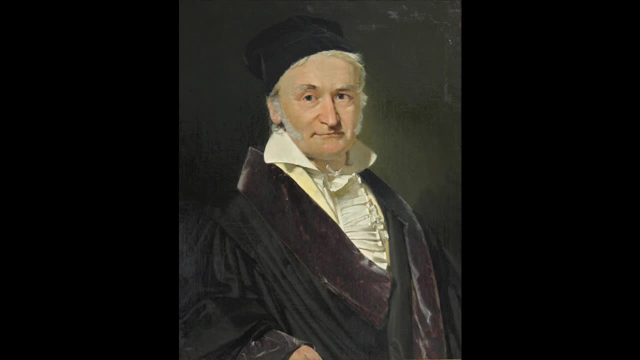 published his method of least squares in 1805 and Gauss shortly after, in 1809, but Gauss had used this method earlier in his study of the length of theよろしく square matrix. It is a more of series. Both Legend and Gauss were able to solve these equations by what they called. 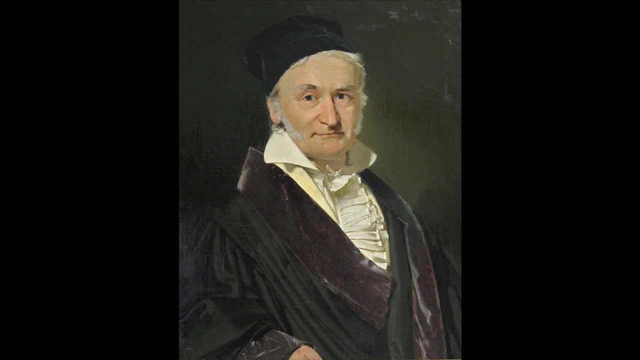 ordinary methods and common elimination, which was understood to mean Newton's elimination method. Gauss made notational changes to the method using brackets to solve least squares problems, and in doing so began the development of so-called professional elimination, which became extremely useful in the increasingly important field of cartography. 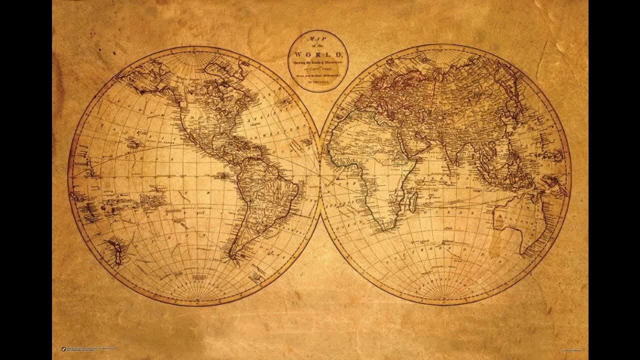 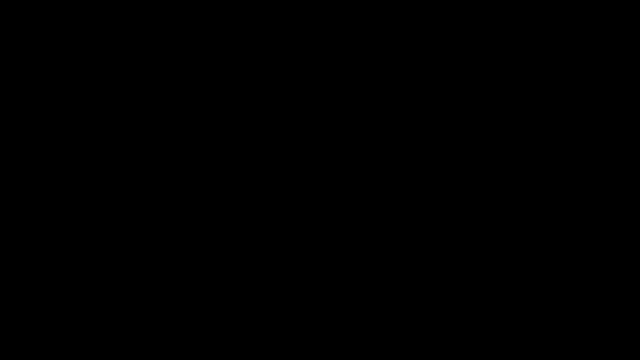 The ease at which it became to solve systems of equations, as well as the development of matrix notation, would set the stage for the discoveries of the mid-to-late 19th century. The next major breakthrough was provided by who you would think to be an incredibly unlikely source. 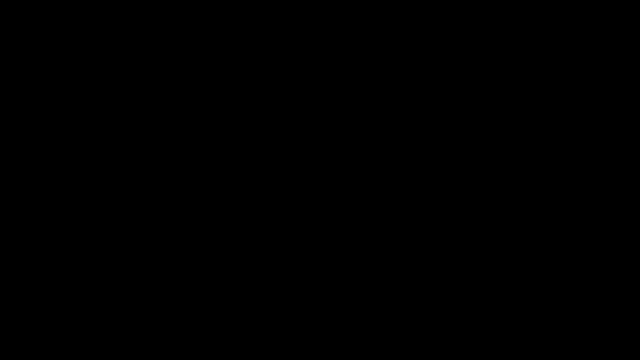 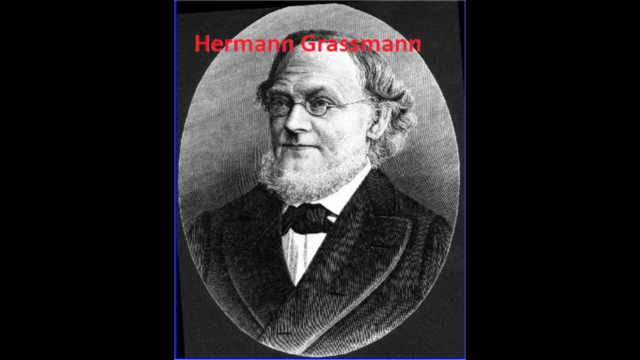 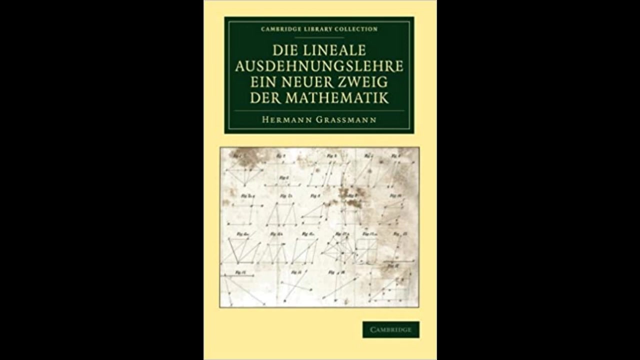 in a German secondary school teacher who was a linguist by trade, a specialist in Sanskrit literature, Hermann Grassmann, published his Ausdehnungslehre, or Theory of Extension, in 1844, which, among other things, furthered the 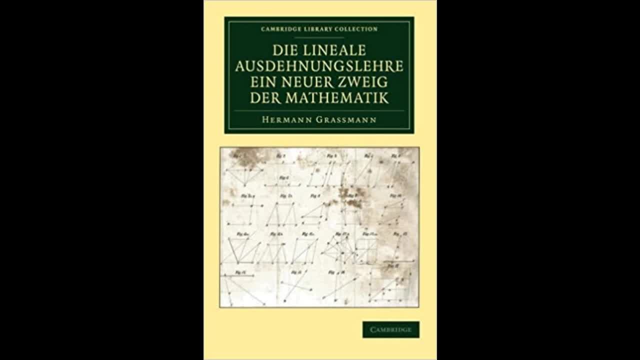 notion set forth by Descartes, that math doesn't necessarily have to be able to be represented in the physical world for it to be meaningful or important. His father, Justice Grassmann, was a mathematician that studied combinatorial mathematics and influenced his idea that math 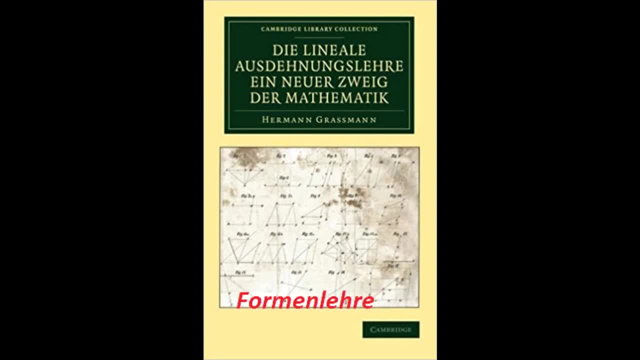 was a science of forms, Which he called Formenlehre, rather than simply a science of quantities. One of Grassmann's most important contributions was his focus on the concept of dimensions and that geometry occurring in two or three dimensions could be considered special cases. 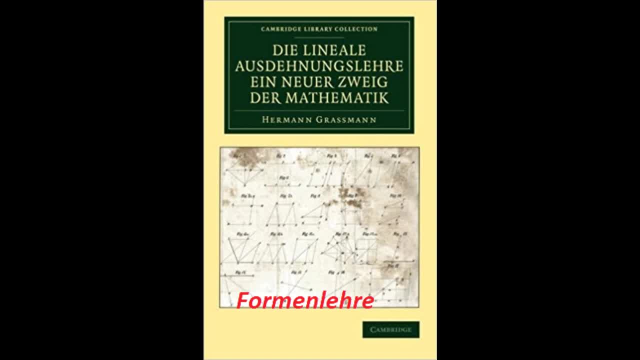 of a more general, abstract view of spaces and subspaces. His Theory of Extension was the idea that math doesn't need to be bound by a single line, but rather that it can be represented in a single line by what the human mind can conceptualize, being limited to only three dimensions and is. 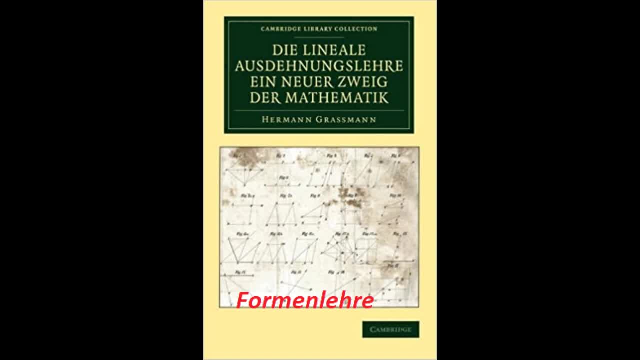 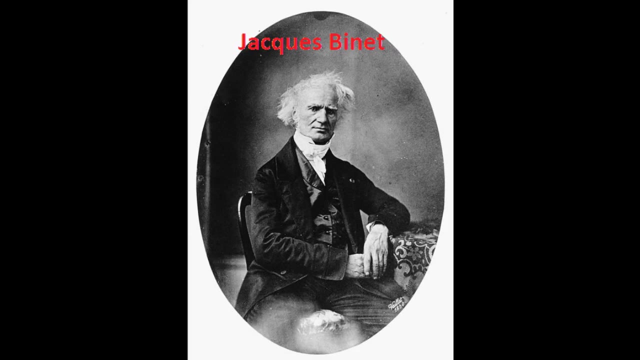 considered the abstract foundation of geometry. He also defined the concepts of unions and intersections that are used in combinatorial logic. in the same text, In 1812, French mathematician Jacques Benet realized that by switching the order in which linear transformations were applied, 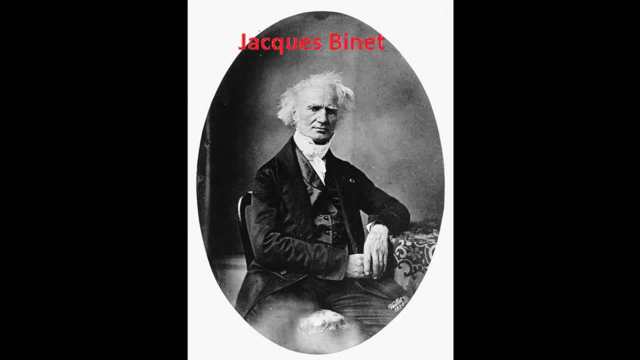 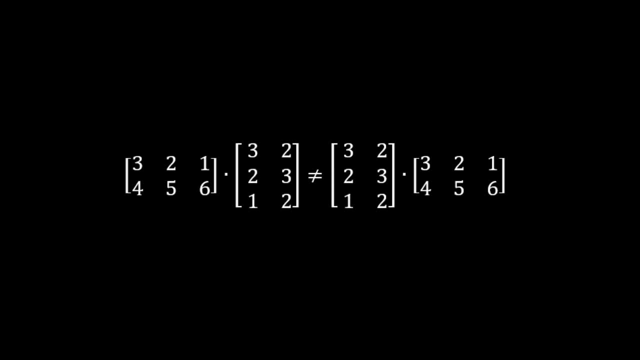 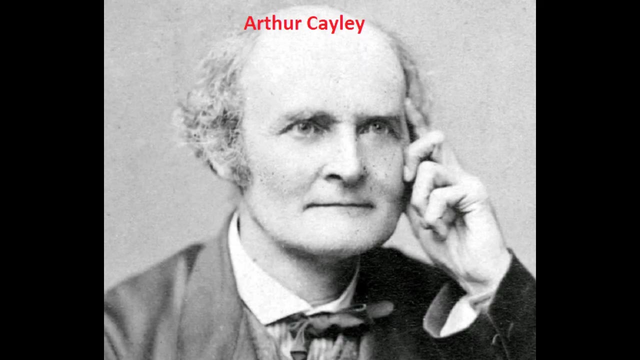 he would get a different resultant transformation. This was the discovery of matrix multiplication, as well as the realization that it's non-commutative. Another major stepping stone to the linear algebra of today was taken by Arthur Cayley. In 1843, Cayley became among the first to study a generalized analytic geometry. He realized that 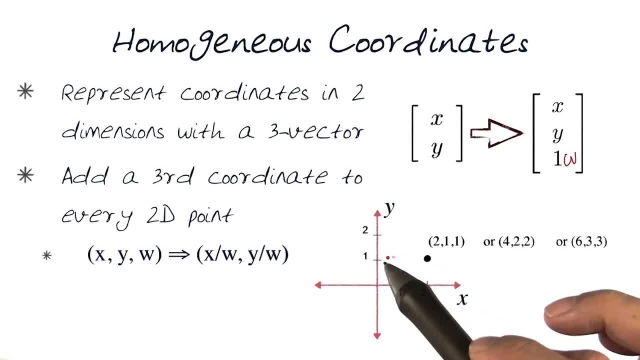 by using homogeneous coordinates, a coordinate system used for geometric projections into a lower dimension. he could represent a fundamental n-1 dimensional element in n-dimensional space by utilizing the determinant, for example, a line in two-dimensional space or a plane in three-dimensional space. He also realized that by expressing formulas for two and three dimensions in the right way, that 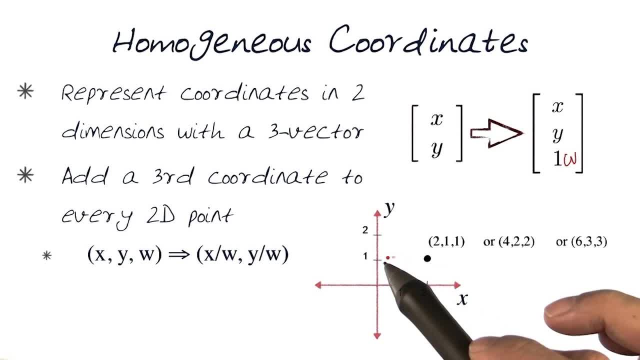 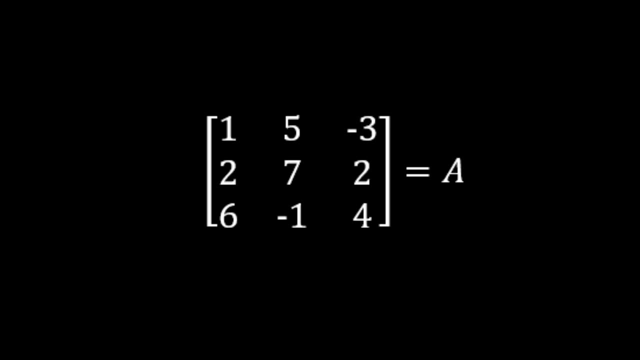 they could be easily generalized to any number of dimensions. This wasn't Cayley's only contribution to the development of linear algebra, though. He was also one of the first to rigorously study matrices, as well as being among the first to use a single letter to represent a matrix, treating it as a single object. 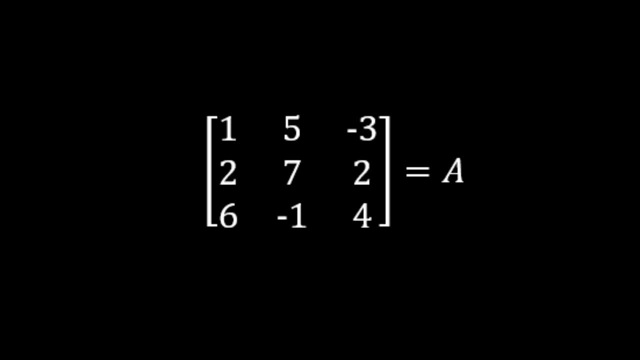 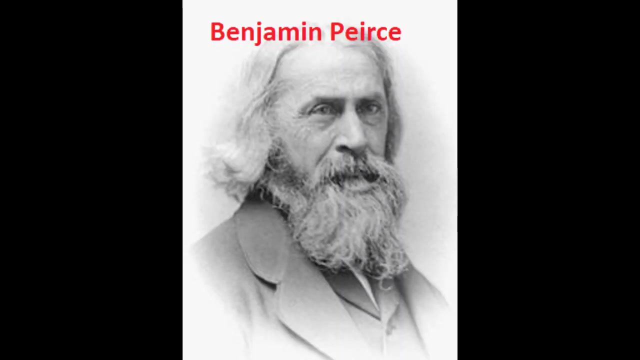 This development, along with Benet's discovery of matrix multiplication, was key in formalizing the algebra of linear systems. Probably the most notable American who made contributions to the development of linear algebra was Benjamin Peirce. He was a math professor at Harvard, where he also graduated from and is known by some as the father of pure mathematics. 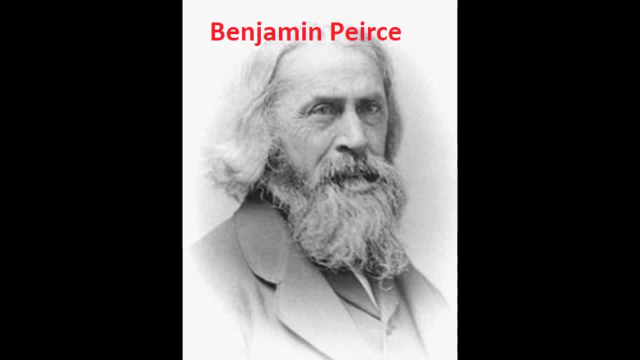 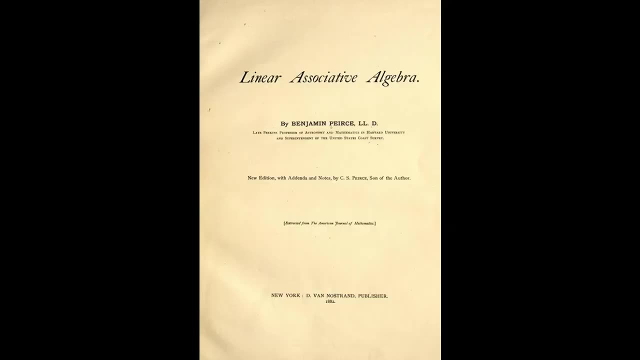 He made observations of Neptune and helped to determine its orbit. but his most notable contribution was the 1870 publication of his Linear Associative Algebra. In this book, which became widely known from its 1881 re-publication, he classified all complex associative algebras up to the sixth dimension. 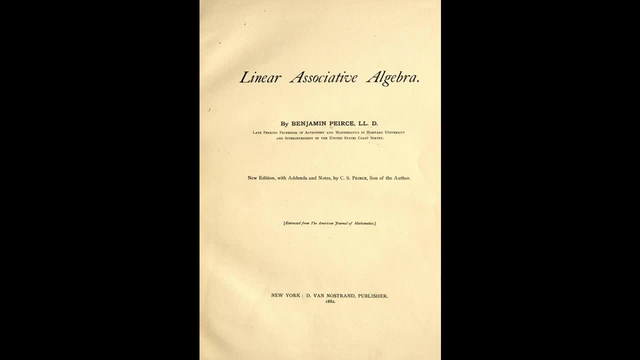 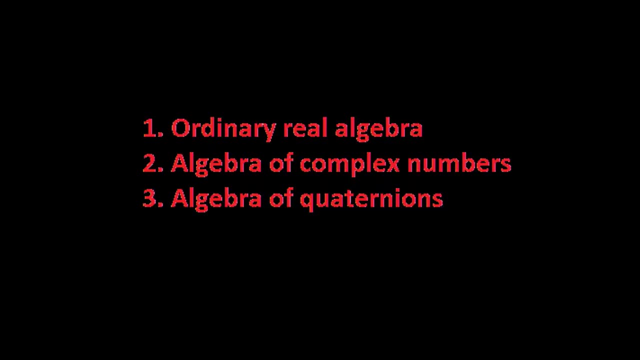 making multiplication tables for 162 different algebras in total and finding that only three contain the property that division is uniquely defined. He formed a general theory of linear associative algebra using terms he created called idempotence, which is a general theory of linear associative algebra using terms he created called idempotence. 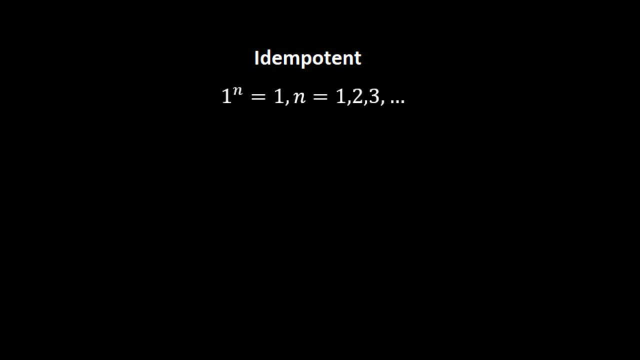 which is a general theory of linear associative algebra using terms he created called idempotence, which is a general theory of linear associative algebra using terms he created, called idempotence, in which an element remains the same after raising it to any positive power. 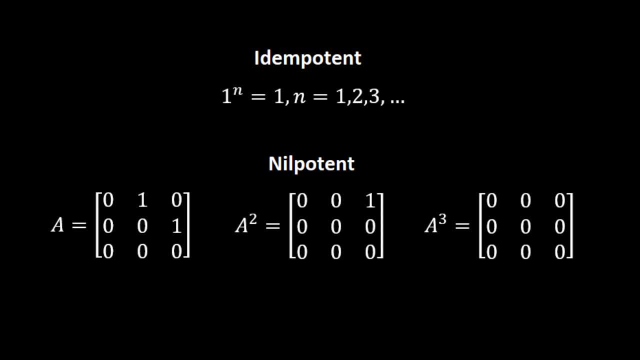 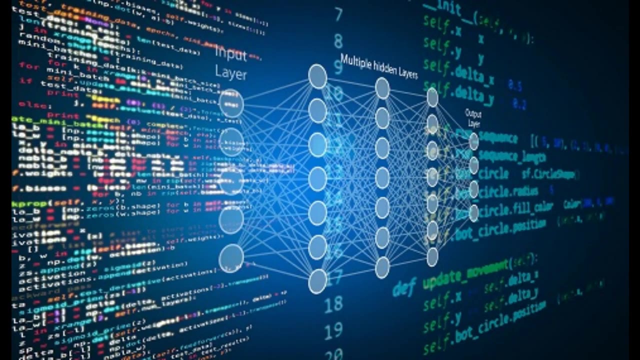 and nilpotence, in which an element raised to a specific positive power equals zero. By the middle of the 20th century, linear algebra had been revolutionized by the advent of computers. Computers are able to find determinants of arbitrarily large matrices and perform Gaussian elimination relatively efficiently. 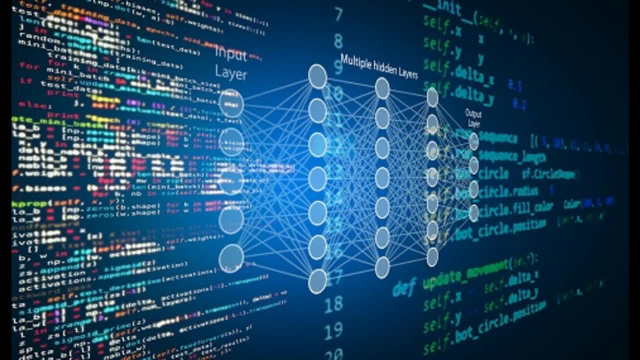 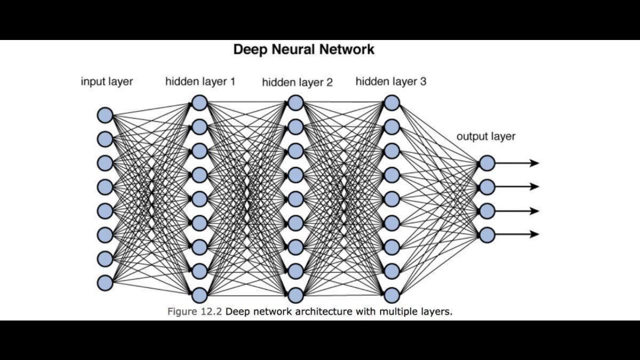 with both having computational complexity. O of n cubed. Fortunately so, because linear algebra is extremely useful today in multiple facets of data science. It's used extensively in machine learning and neural networks, in which a program is given a data set to learn from. 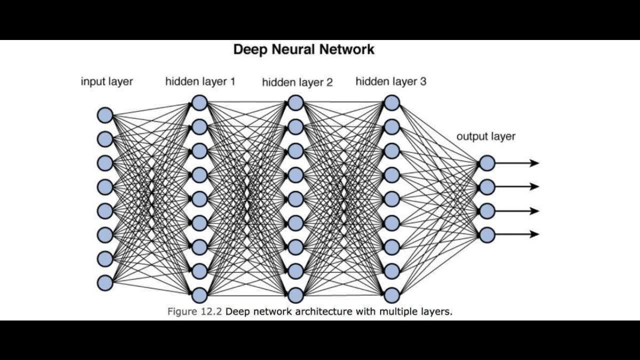 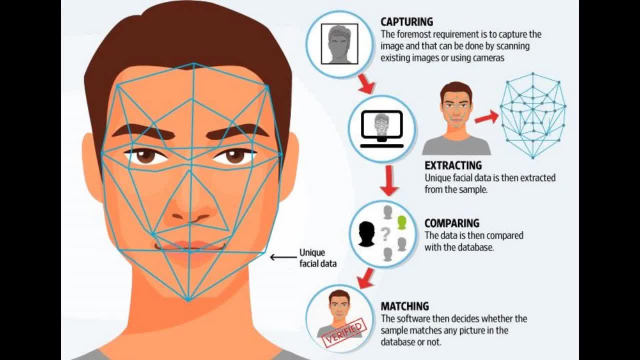 and afterward will be able to predict or determine future problems given to it. This can be used for a variety of applications, such as facial detection and vertebration analysis and recognition, image recognition and sound recognition, The algorithms used for recommendation systems and search result systems, such as those found on: 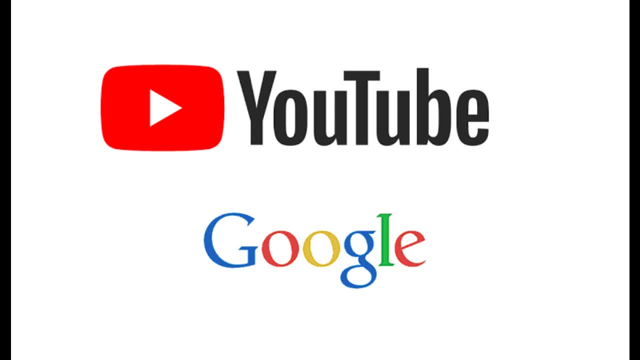 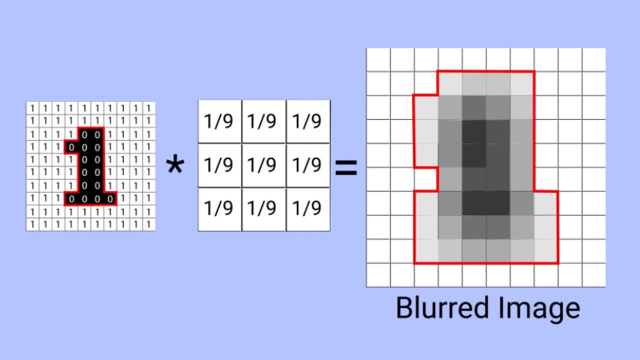 YouTube or Google use linear algebra to determine what videos or websites are the most useful or relevant to a given search. It's also used in image editing. A convolutional matrix called a kernel sweeps across an image and changes it based on how the kernel is weighted. This is how visual effects such as blurs 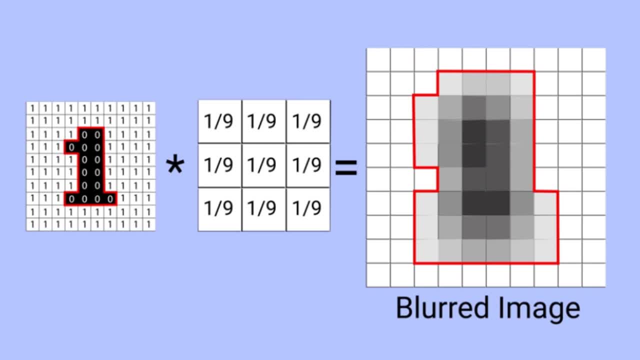 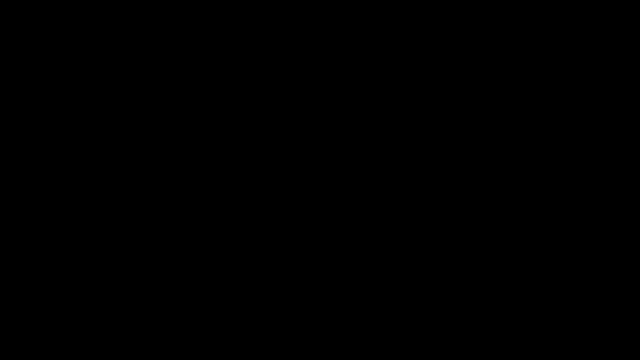 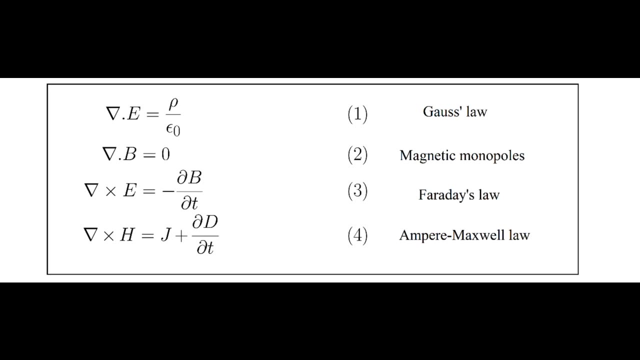 and edge detection work. Linear algebra is also at the core of quantum computing and computer graphics. In physics, any topic that deals with vector fields can be represented using a matrix. Maxwell's equations, for example, deal with vector fields that change over time, and the vectors can be organized into their own. 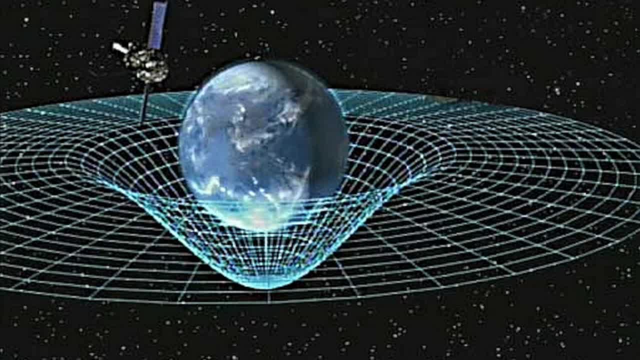 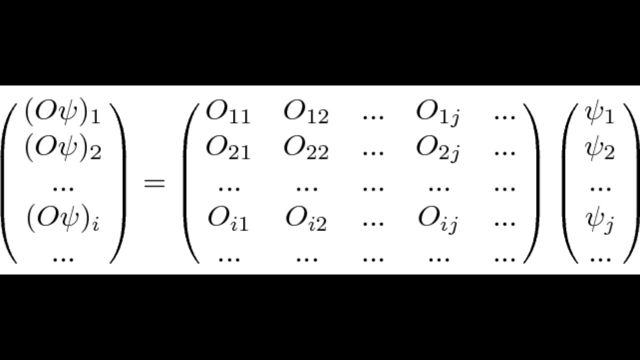 rows in a matrix. The theory of relativity uses the transformations of distance and time by mapping those vector spaces into a matrix. In quantum mechanics, physical variables are represented by operations on the wave function and are usually linear equations. This linearity means that we can use linear algebra to 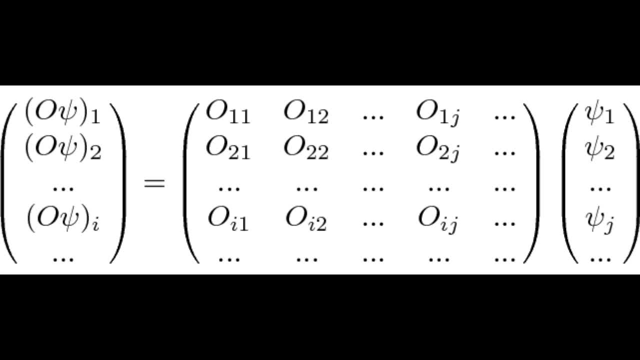 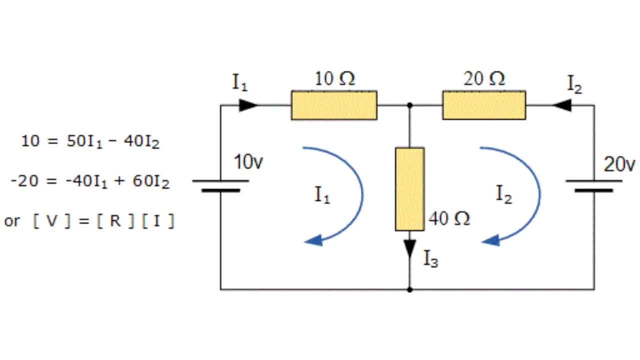 calculate how those operations act on the vector space. Another extremely common and useful application of linear algebra is the use of linear algebra to calculate how those operations act on the vector space. Linear algebra is an electrical engineering and circuit design. Not only do circuits need to perform their designated 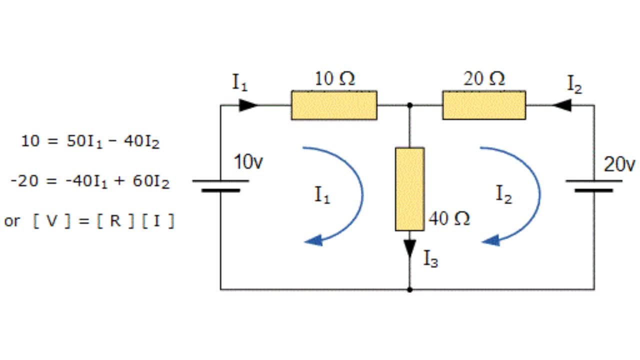 function, but the individual components have to follow certain tolerances that are allowed by each of them. Large circuits become extremely tedious to analyze and reduce, and so the voltages, currents and resistances can be put into a matrix, which can then be solved. 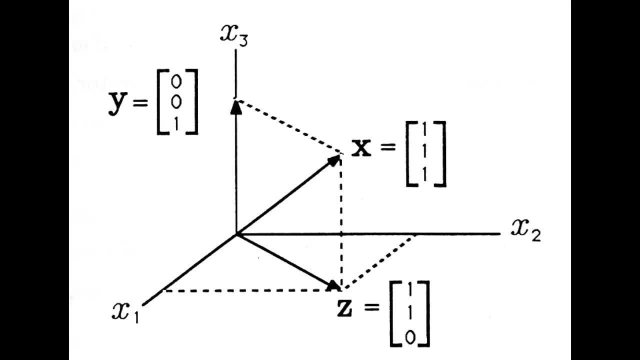 with Gaussian elimination. Linear Algebra is a very common and useful application of linear algebra. It can be used in many ways and can be used in many different ways. Linear algebra is a very common and useful application of linear algebra. Linear algebra is a very common and useful application. 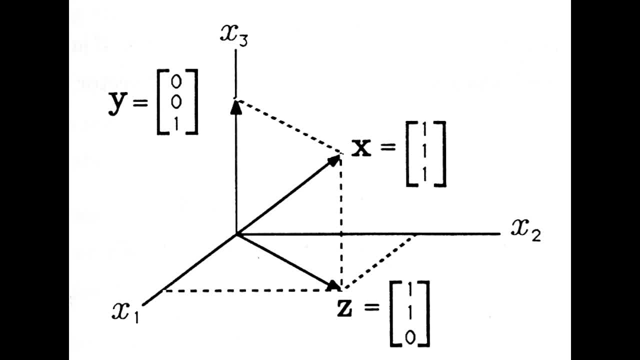 that can be used in many ways, and can be used in many different ways. Linear algebra is a relatively new field of mathematics, only being rediscovered around the same time that calculus was being developed, but it has proven to be incredibly useful in various fields. 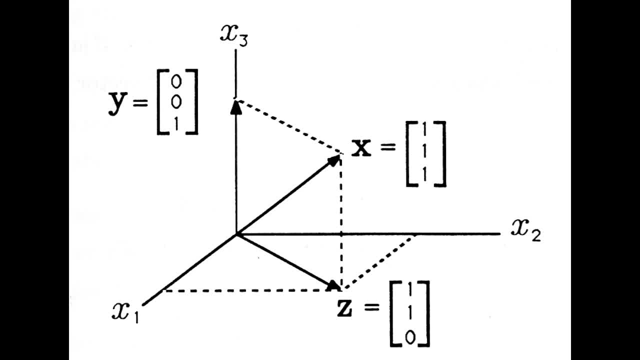 over time. Much of our lives today are built on foundations of linear algebra and the ease at which computers are able to solve and perform calculations on matrices, even though most of us don't even realize it, and I think it'll be interesting to see where it can take us.